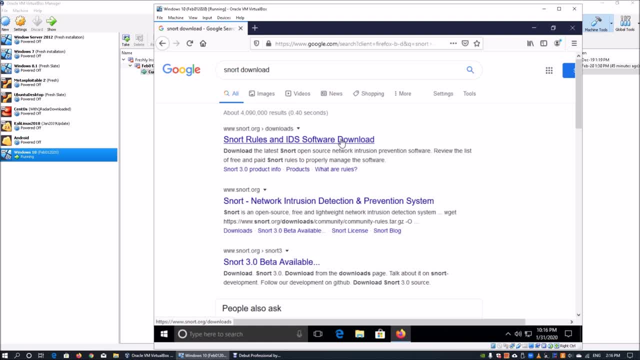 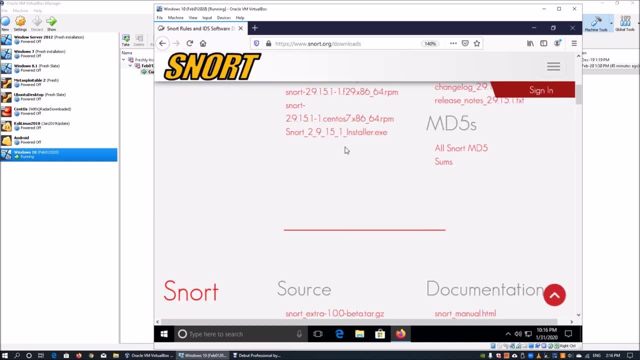 you can actually go into the first site, which is snortorg. So once you're in you can actually scroll down a little and you can zoom in to the binaries. and in the binaries you can see there is a snort29151installerexe. So click on that to go ahead and download this executable. 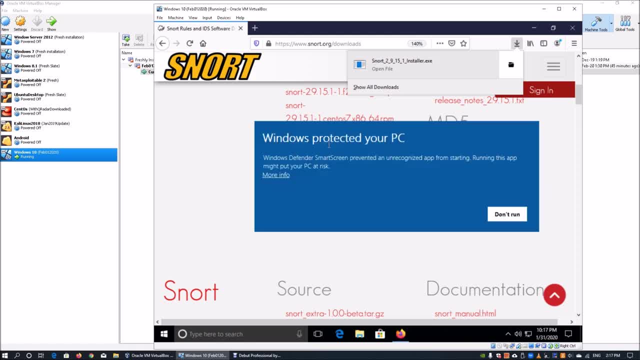 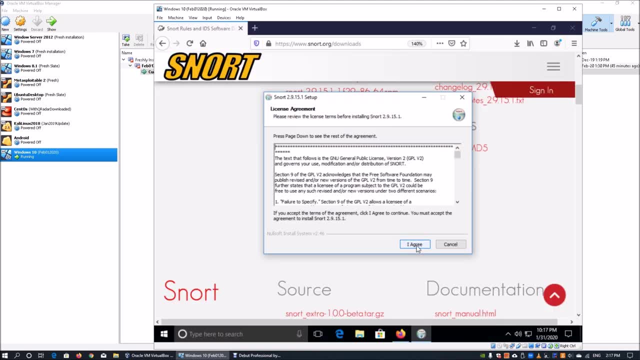 So once we're downloading and we have the executable running, so what we can do is we can go ahead and run anyway. So this will help us install snort into the operating system. So of course you can read through the license agreement and once you click, I agree there. 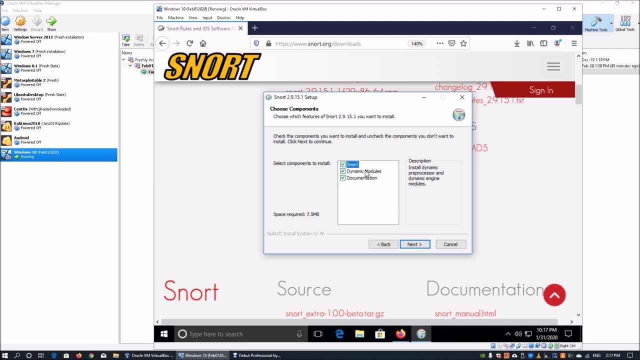 are three key components, So one is snort itself, which we can also move on into the dynamic modules, as well as documentation, which has some of the key information, And once you're done you can go ahead and click next. So we will install it directly into the default. 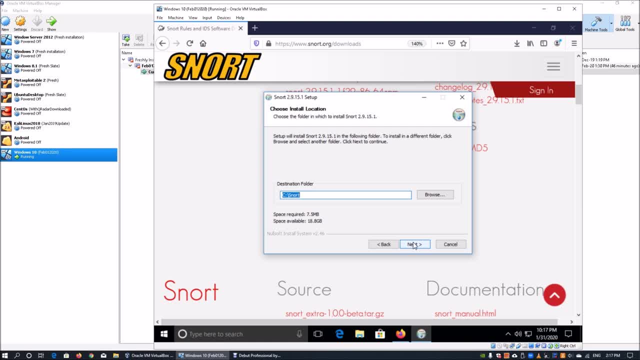 folder which is c drive slash snort And this will only require a little bit of time, So let's go ahead and go ahead and click next. Last two Forever 6 transactions will require 7.5 megabytes, So click next on. 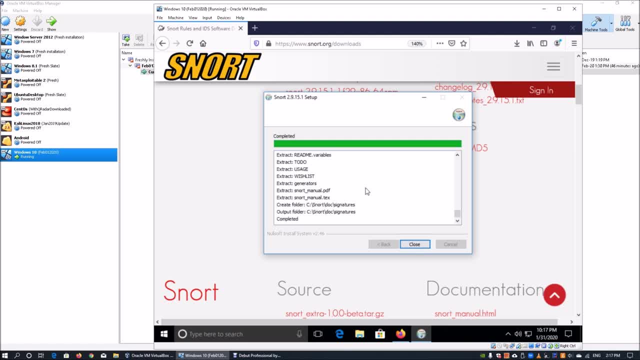 that and installation will be completed very quickly And of course, you can show details to see what are the things that has been generated on and so on. So you see a creation of folder, you see that creation of binaries beam And then as you scroll down, you can see poly pues & preprocessing rules and so on. So once you're, 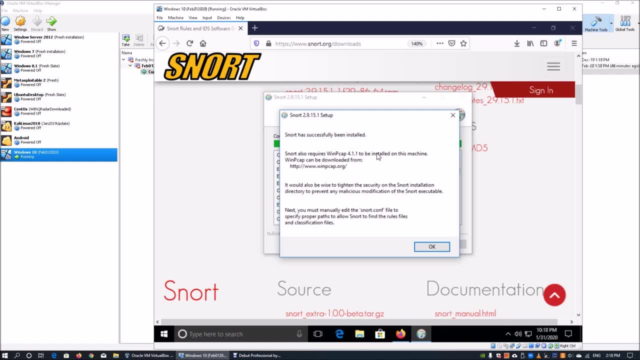 done, then click close on that And it pop up. Solid好的 Brings you up and say that we require snort Sidmb4.1.1 to install on this machine. So the only way that you must inspire us is using the standard b Spencer validation package andombres, which is an RCD. 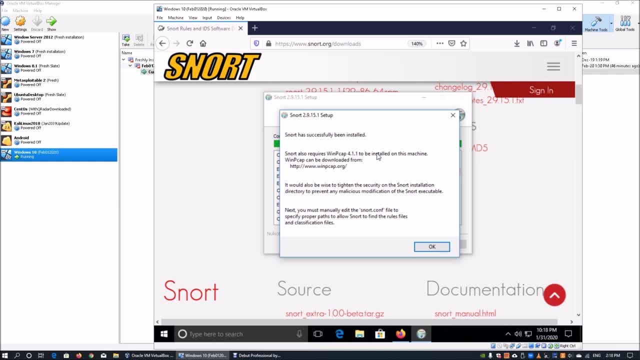 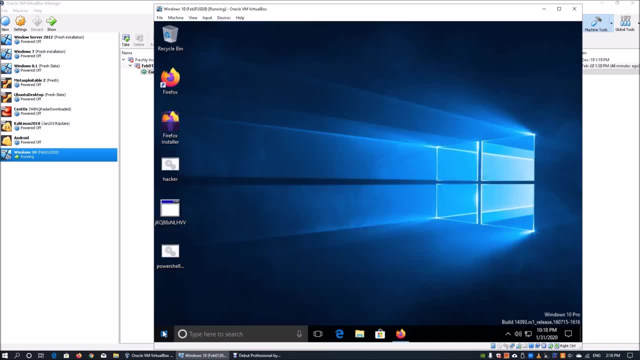 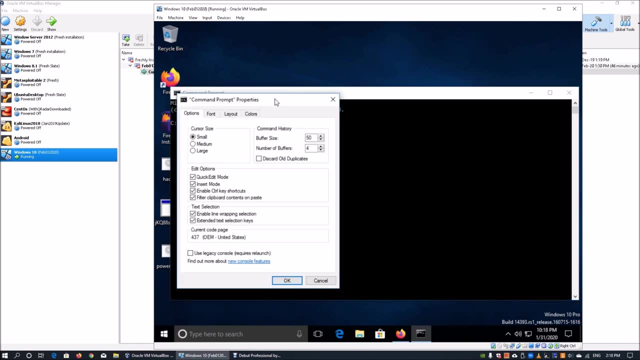 OKдержji install this in order to get the intrusion detection system running. So click OK on that and of course from here we can actually go into terminal So you can go and enter cmd, and once you're in cmd we can actually adjust the font size so that you can actually see. 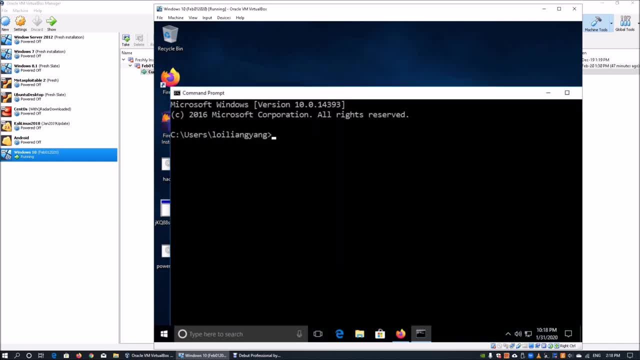 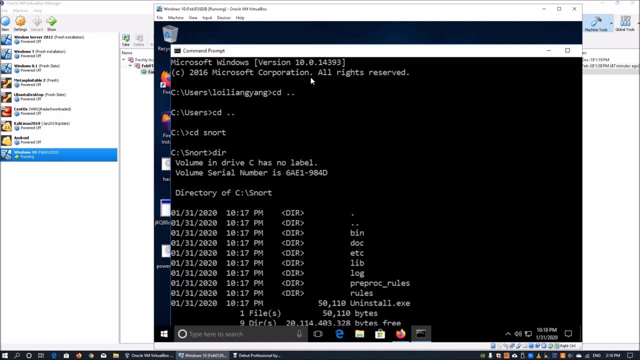 more clearly. So we'll use the font of 24 and of course we can cd dot dot, We can go into c drive and we can cd into snort and we can enter the ir. So this is the directory of snort and of course, 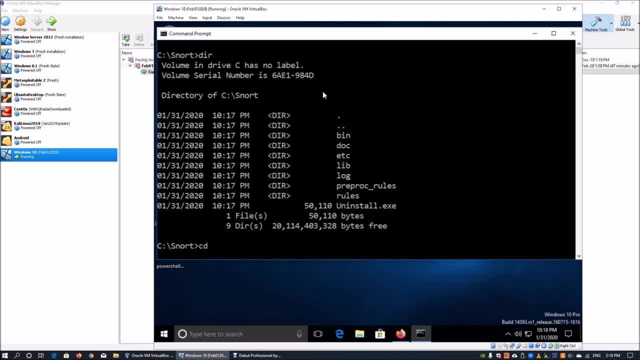 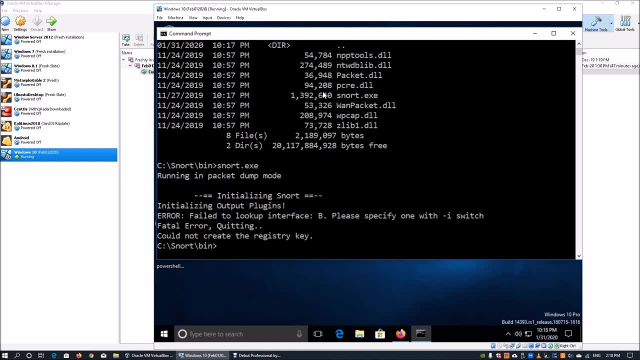 in the directory we can see a lot more information and we can cd into bin. So this is where all the binaries are being kept at, and if you enter snortexe, you will realize that you get a failure because we do not have a WinPCAP installed. So go back into your favorite browser and this time, 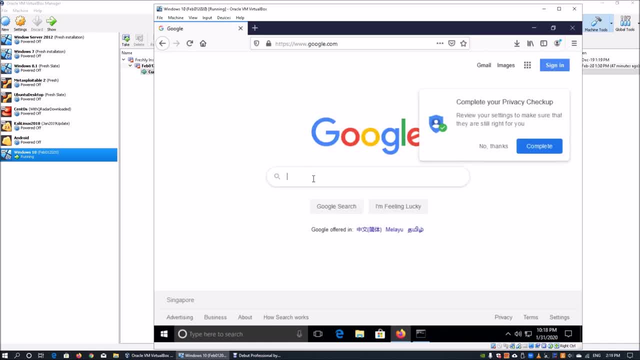 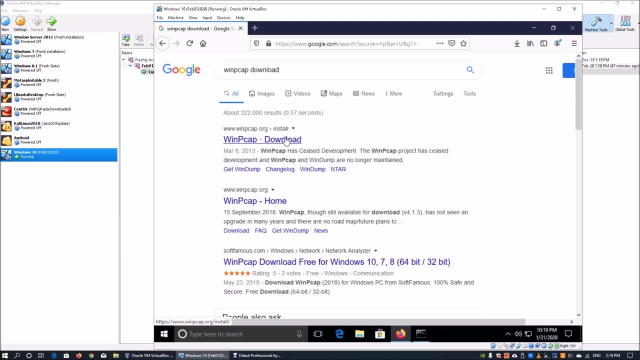 around. we are again going back to your favorite search engine and we are going to enter WinPCAP download. So once you do that, again we are going into the first page or the first result coming out from the search, so which is WinPCAP. 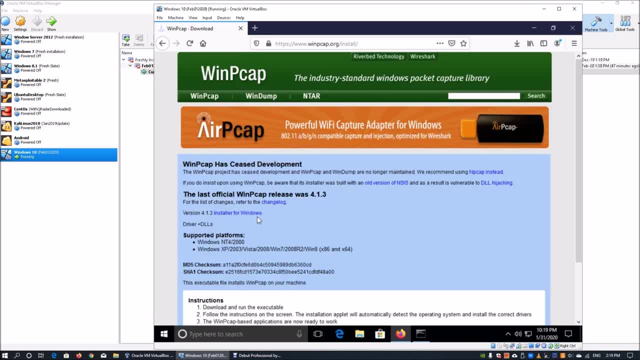 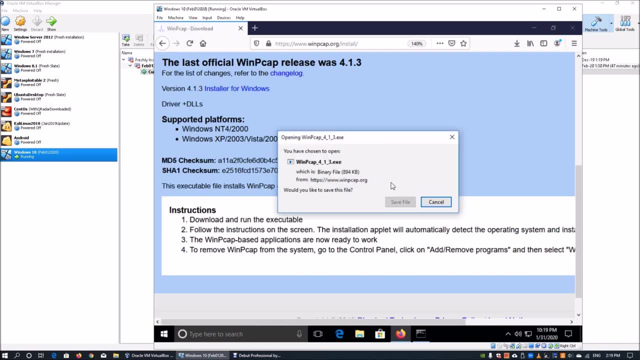 download, So winpcaporg. click on it and of course here we have a key information and it says installer for windows. Click on installer for windows. so likewise it will say save file, so we can save down the file into your system and once the download has completed, you can click on WinPCAP. 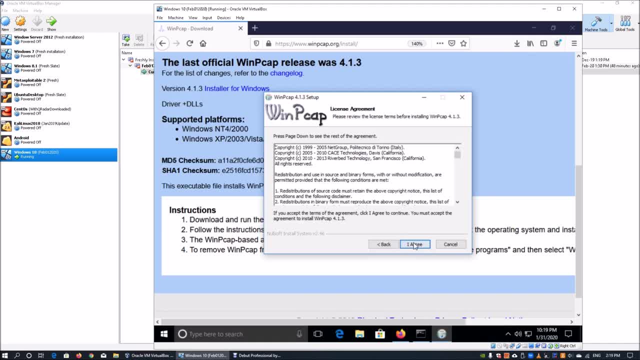 and we can install it. So what we see here is the setup wizard and of course, you can read through the license agreement too and click I agree and, of course, automatically start the WinPCAP driver at boot time, Click install and, once the installation is completed, what we are going to do, 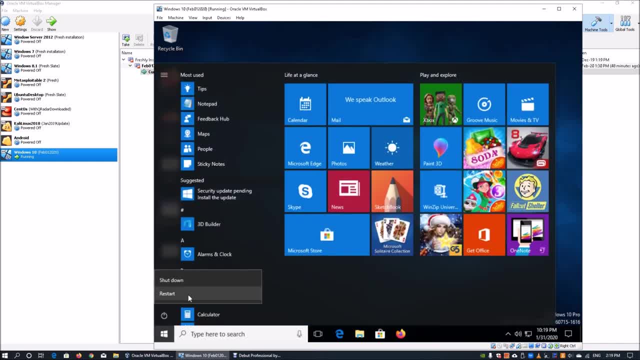 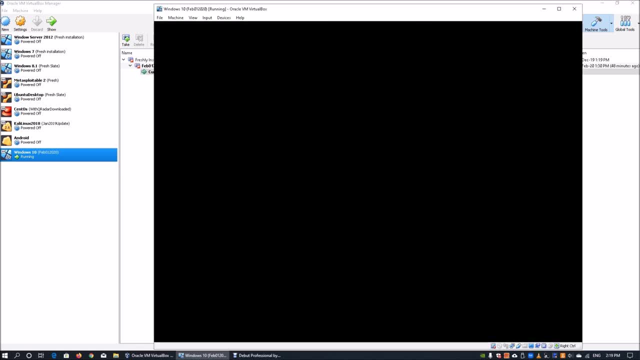 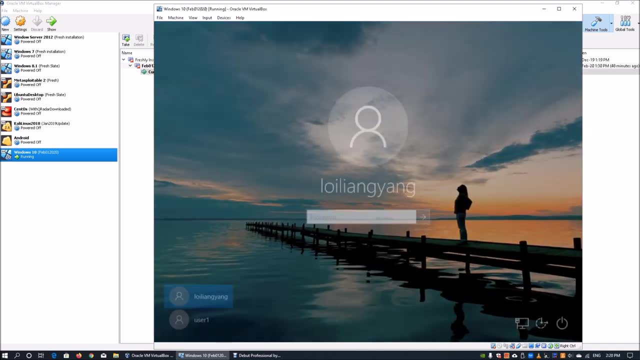 right now is we are going to restart the computer so to ensure that all the drivers and all the information is being installed properly into the operating system, and then we'll be able to start intrusion detection system very quickly. So now we are back up into the operating system and we can 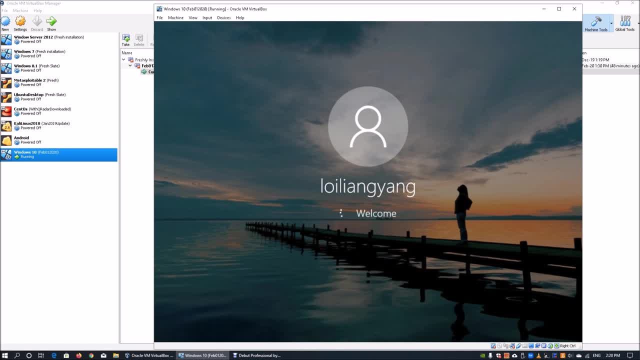 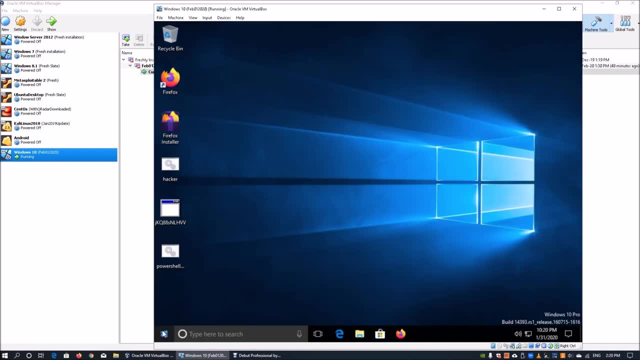 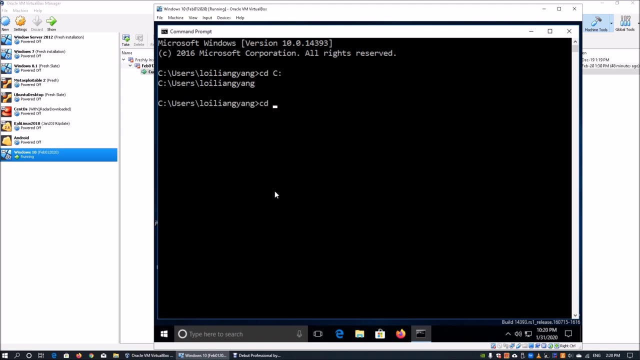 go ahead and log in, So of course enter your password once more. so right now we got both snort as well as winpcap. So with it installed, right now what you can do is you can actually go back into cmd, which is command prompt, Launch, command prompt, cd, into c drive or what from there on we can. 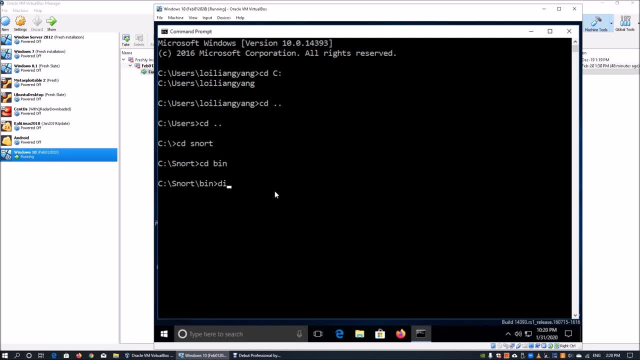 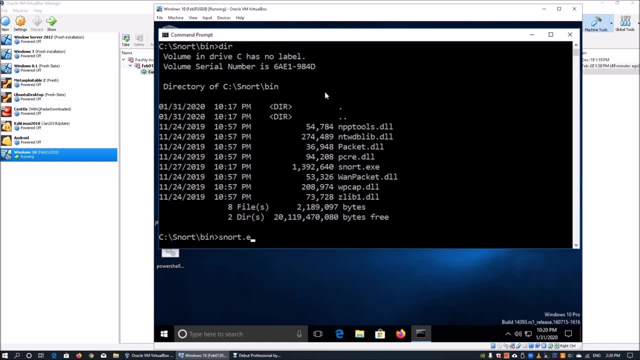 actually go into snort and cd into bean and then do a dir and we're going to use this chance to actually launch the snort executable So we can go and enter snortexe. and once you do that, we see that on top. we got all the information running. so we have all the information running. So we have all. 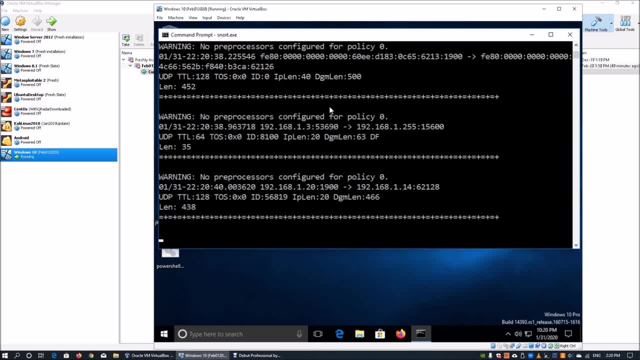 the packets details that are being pushed out and we can see what's being transacted and, of course, this will actually help us complete the setup: the installation and setup of snort, which is an intrusion detection system on your windows operating system. So there, you've seen it how.